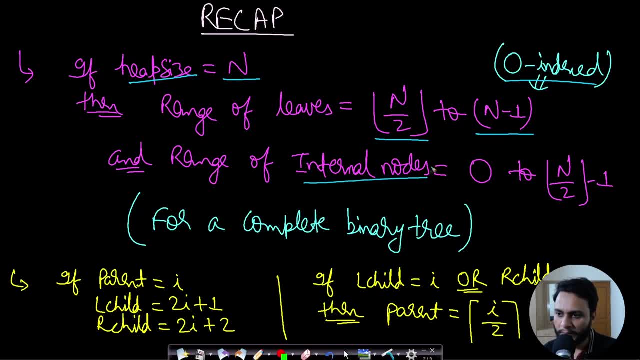 zero, indexed Okay, and the range of internal nodes will be the rest of the nodes. The nodes which are not the leaf nodes will obviously be internal nodes and therefore it will range from 0 to n by 2 floor minus 1.. So this is true for a complete binary tree. Now, if our parent is at index i, then the left. 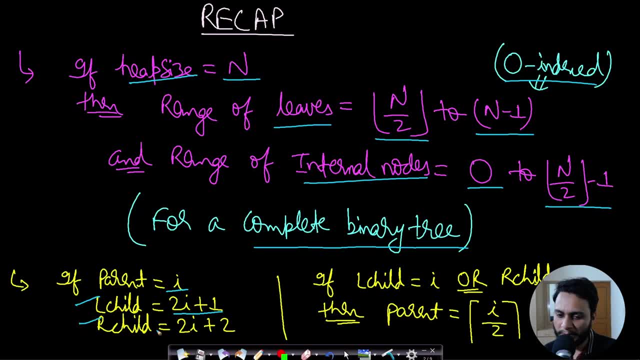 child will be at index 2 into i plus 1 and the right child will be at index 2 into i plus 2. and similarly, if our left child is at i or our right child is at i, then our parent index will be i by 2 seal minus 1.. 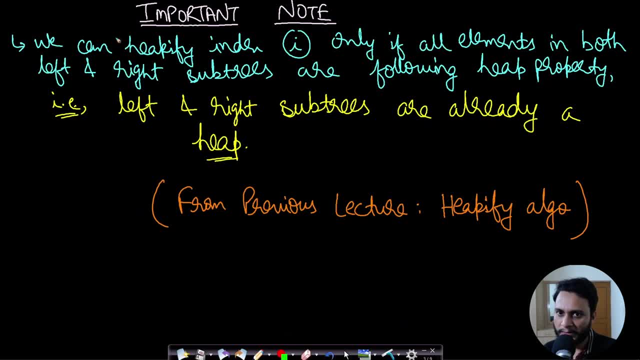 Right. So this was just a recap. Now, one thing to note here is we can heapify index i only if elements in both the left and the right subtrees are following the heap property. that is, the left and the right subtrees must already be a heap, okay. so this I have already explained. 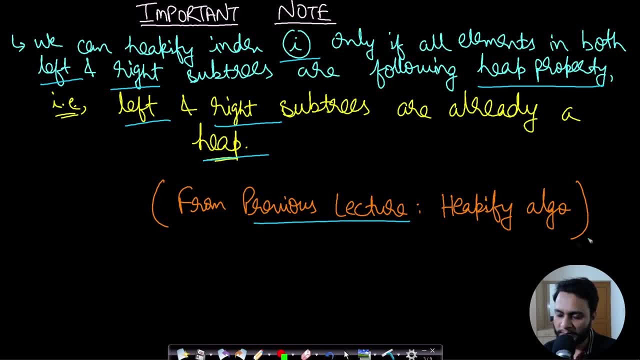 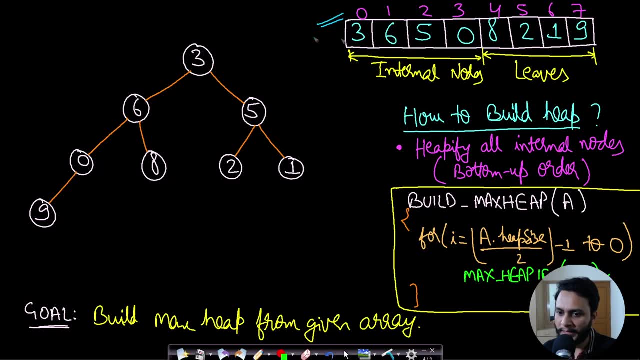 in the previous lecture. the link for that will be present in the description below. Now let us see: if we are given an array, then how do we form a max heap out of it? okay, so our goal is: given an array, we want to build a max heap. okay, so let's assume that here. 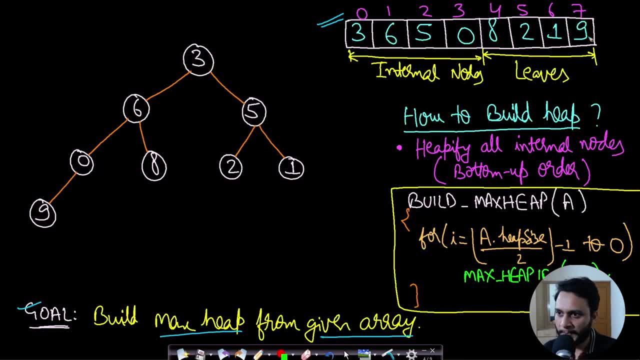 we are given 8 elements in the array indexed from 0 to 7.. Now we can easily find out the range of leaves according to the formula which I had shown. okay, and the rest of the nodes will be the internal nodes. Now, having known that, I have already told you that the leaf node will always follow. 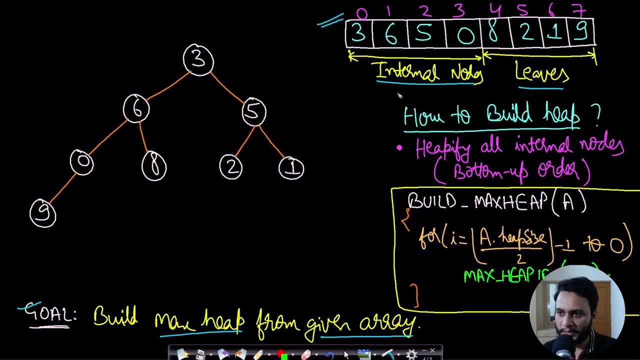 the heap property. either you talk about the max heap or the mean he property, it will always follow the heap property, right? So the only nodes which we need to take care is the internal nodes. Now, if we just heapify the internal nodes, then our entire array will now become a heap, okay, 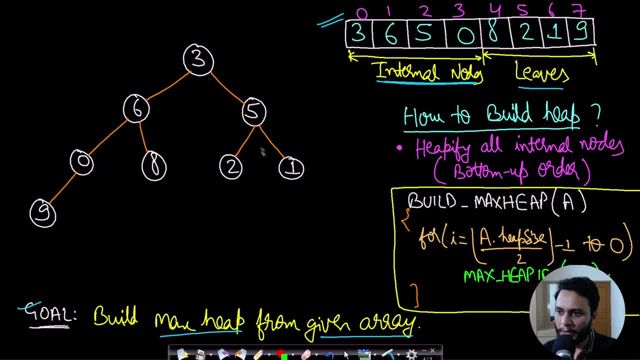 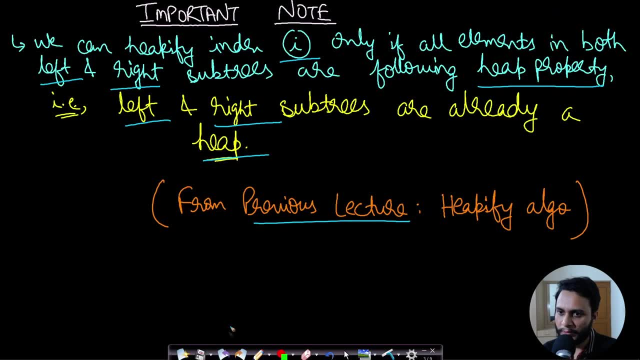 so let us max heapify this entire heap. now, how do we do that? in what order should we heapify? okay, so that is a very important question. Now in this case, I had already shown in the important notice that if you are applying heapify on index i, then the entire left subtrees as well as the entire right subtrees should. 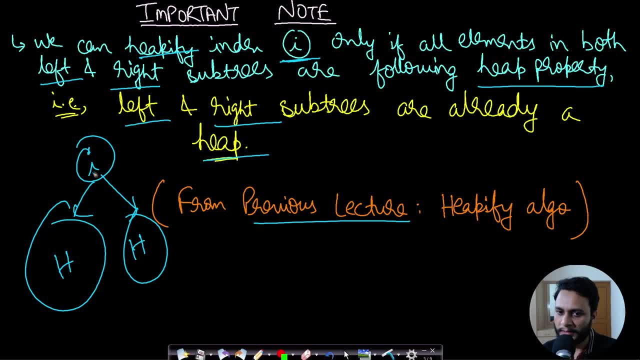 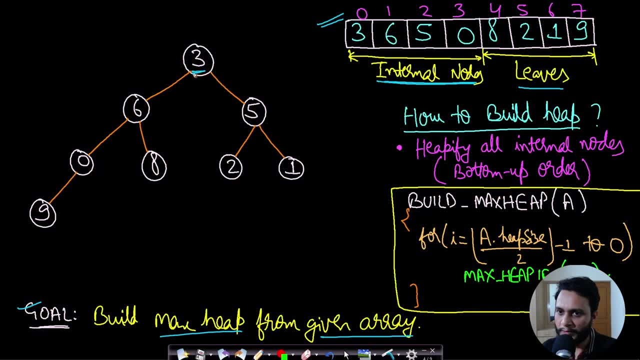 already be a heap. Okay, otherwise you cannot apply heapify on this index. i. so if you know that that concept already, and lets say you want to apply heapify to this node, this is the root node. ok, so lets assume that you are applying heapify to all these nodes from left to right. 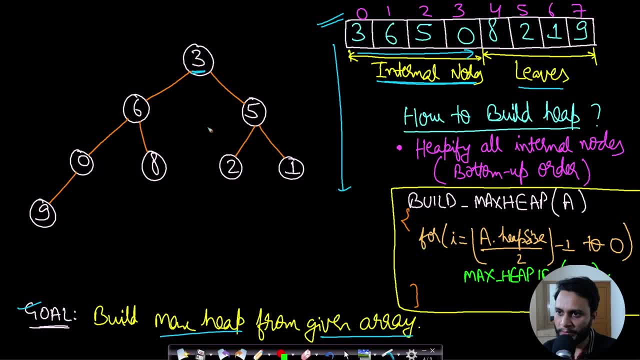 So this left to right is nothing but the top-down order. Okay, So can you apply heapify to this node 3 now? in order to apply heapify to this node 3, this entire left sub tree, as well as this entire right sub tree should already be a heap. okay, but 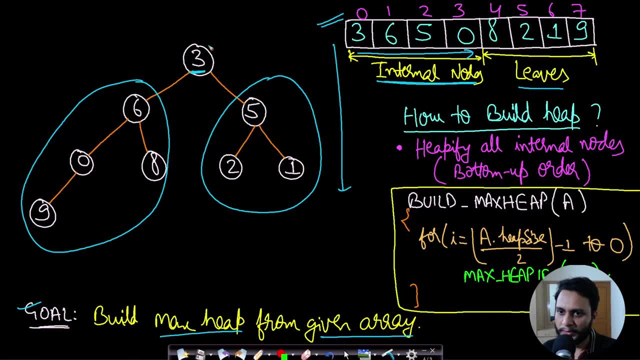 according to this given problem, when you are considering this root node, then there might be some internal nodes in the left sub tree as well as in the right sub tree, so they might not be in order already. okay, so that is why we already know that only the leaves will be following the heap. 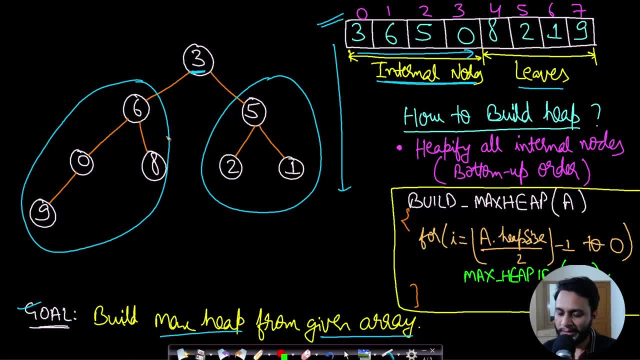 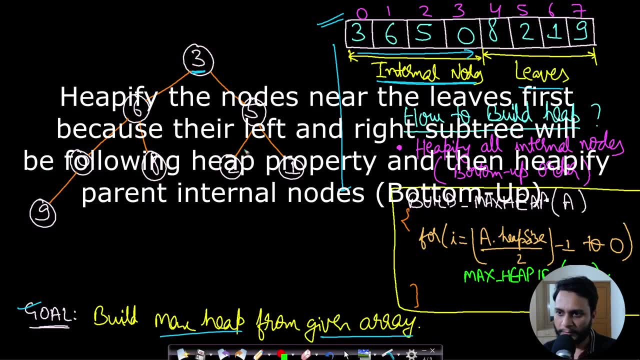 property and not the internal nodes. so we need to first bring the internal nodes to follow the heap property and then we can heapify this element right. so that is why we will have to first heapify the last internal node, that is, this zero, okay, and then we will have to move in the bottom of order. 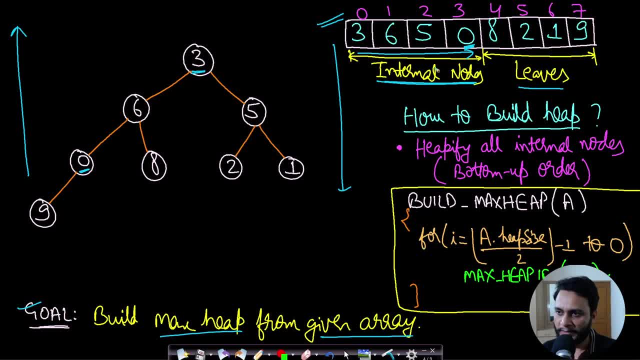 so in this array we will not be heapifying from left to right, but instead we will be heapifying from right to left. okay, now, when we are looking at this zero, this node zero, then obviously this node zero will only be having the leaf nodes, because this is the last internal node, right? 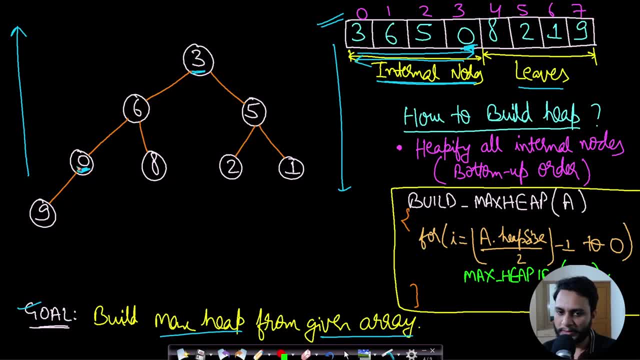 so. So we can apply the heapify algorithm because, since we already know that all its left as well as right child will be a leaf, So they will be a heap. Okay, So now let's compare this nine with zero. Since we are trying to form a max heap, therefore, we will be taking the maximum element. 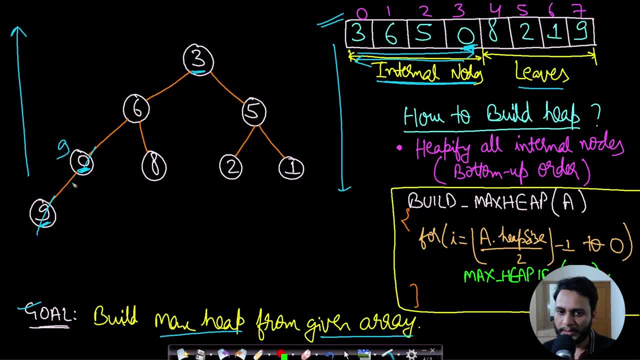 to the root. So maximum is nine. So nine will be replacing the zero. Okay, So there is no right child. It is now heapified. Now move on to the next element. This three index is done. We will move to index two, which is five. Now, at this five, is there any element which is greater than? 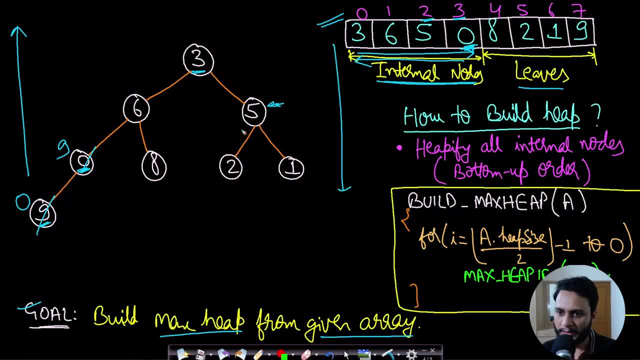 five in the left as well as the right child. No, there is no such element. Therefore, this is already heapified. Now we will move to the next index, which is index one. So at index one, this is value six. Is there any element which is greater than six as its left child or right child? Yes, 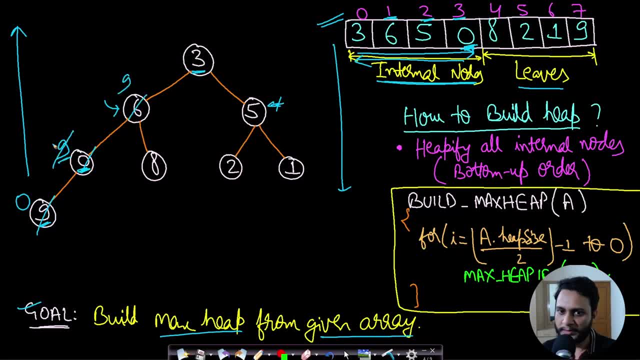 the maximum element is nine, So this nine will be replacing this six. Eight was also greater, but we will be taking the maximum element. Now we will see that this six is already greater than zero, So no need to heapify this one, Okay. 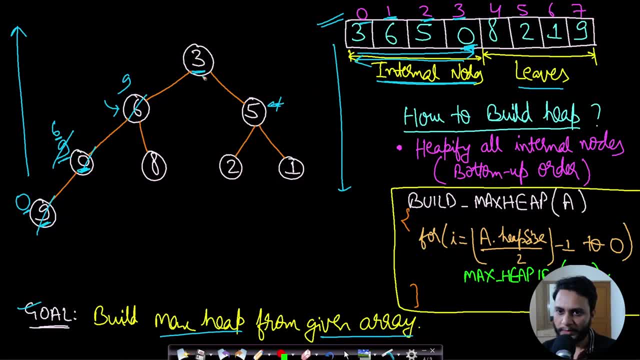 Now we will move to the next node, which is zero. So zero is this one, three Now in its left child, as well as right child, which one is the maximum element. Well, maximum of three comma nine, comma five will be nine, So nine will come here and three will come here. Okay, Now we again need 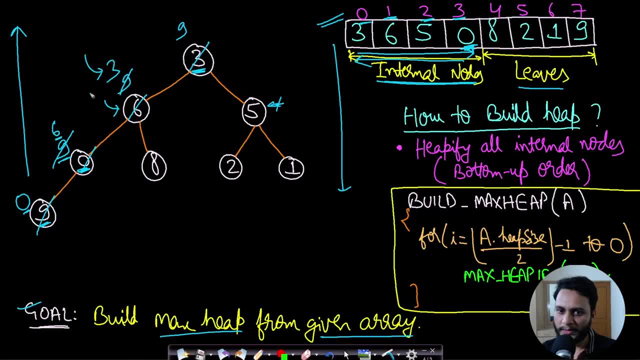 to heapify this. we need to check if this is at the correct place, So in the left child as well as in the right child. which one is maximum? Eight is maximum, So eight will be replacing this value. three and three will come here. Now, three is already a leaf, So nothing. 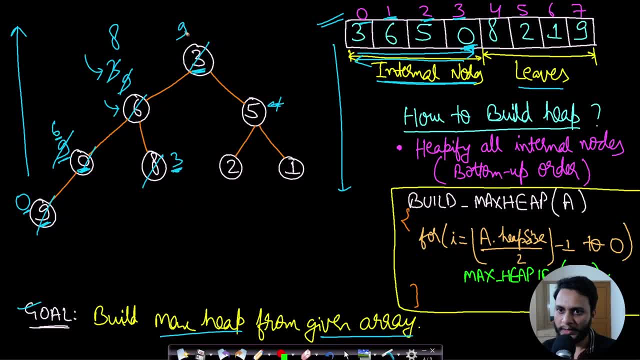 will be done. So this is the final heap structure where nine is forming the root, Eight is its left child, five is its right child And for this node, its left child is six and its right child is three. Okay, and this zero is the last element. So this is the entire algorithm for forming. 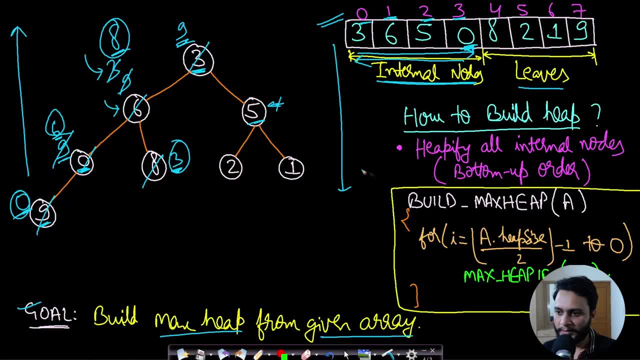 our max heap using the max heapify algorithm. So if you just look at this algorithm in order to do max heapify, what we are actually doing is we are taking all the internal nodes. this, a dot heap size, is nothing but the value n, which is the number of nodes in the array. So we are moving. 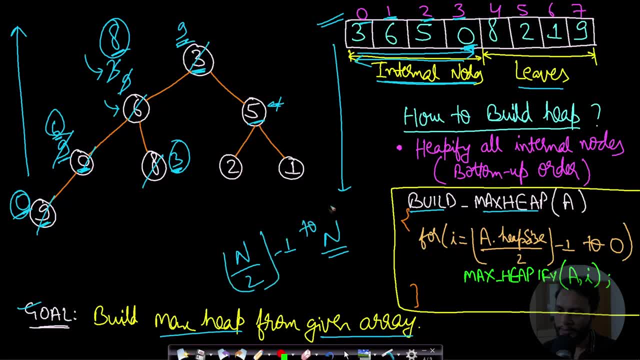 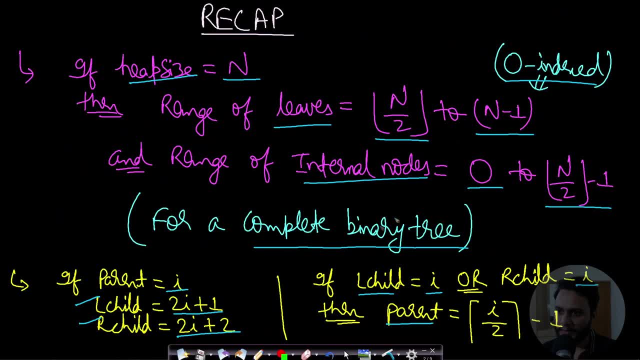 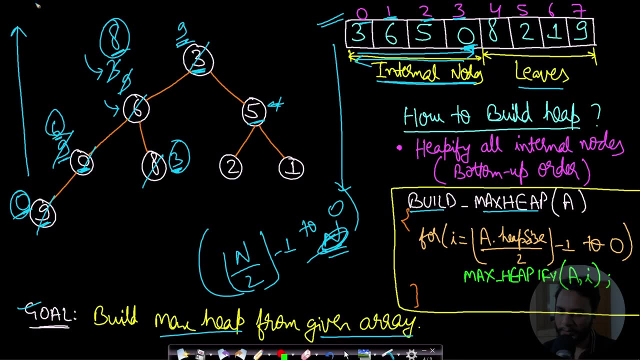 from n by two floor minus one to zero. So this is nothing but the range of our internal nodes. So range of our internal nodes was nothing but, if you already remember, from zero to n by two floor minus one. So we are moving in the reverse order, that is, in the bottom of order. 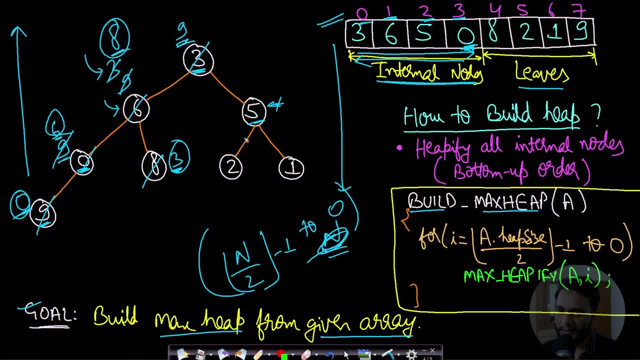 because we cannot heapify a given index i if it's left as well as right, subtrees are not already a heap, Okay, so that is the reason we want to make the lower parts as heap in order to heapify the upper nodes. Okay, So I hope you have already understood this, and this is the max heapify. 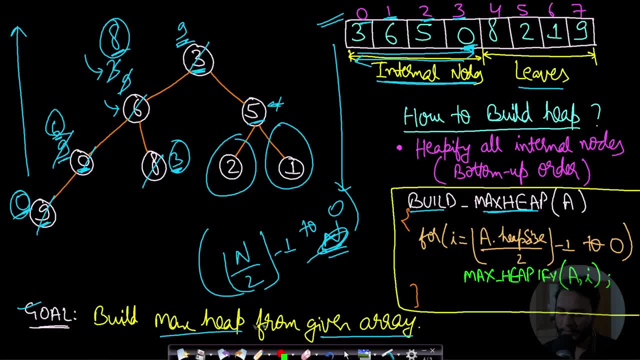 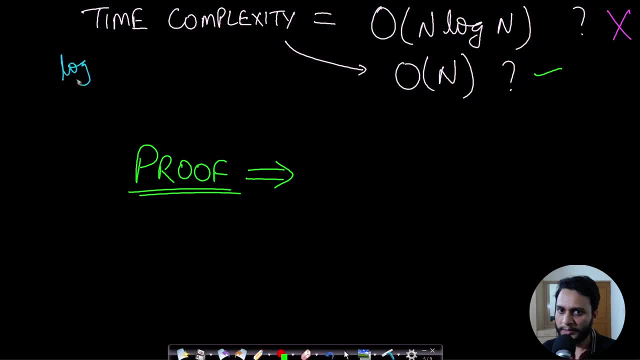 algorithm. we will be heapifying all the internal nodes one by one. Now, once you understood this, what will be the time complexity? you already know that in order to heapify, you need time of log n, which is the height of the tree, because in the worst case you 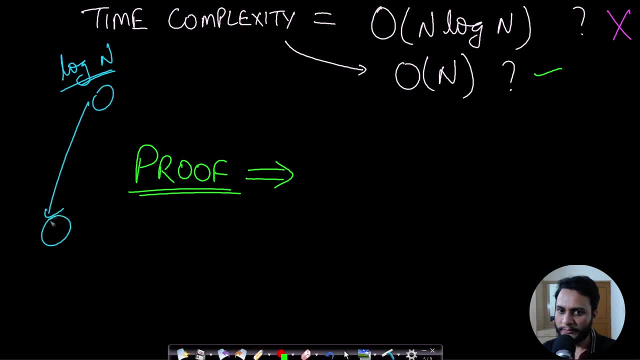 will be moving from the node to the farthest leaf, and that will be nothing but the height of this tree, which is log n. And we are doing this operation for all the internal nodes, and internal nodes are in the order of n by two. So this is nothing but n. Okay, If you. 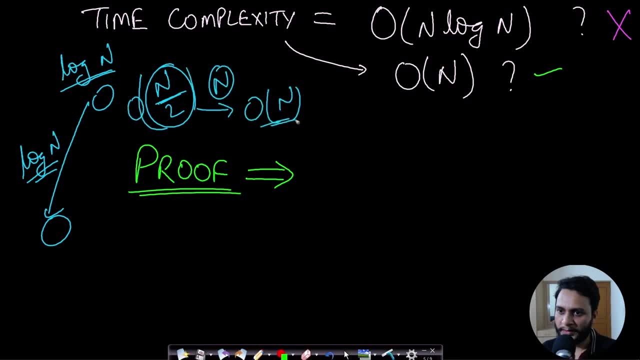 take order of n by two, then this will come as order of n. Therefore the total time complexity will be order of n log n. This seems pretty logical, right? But this is not the case here. The actual time complexity is just order of n. So just for understanding how it is coming. 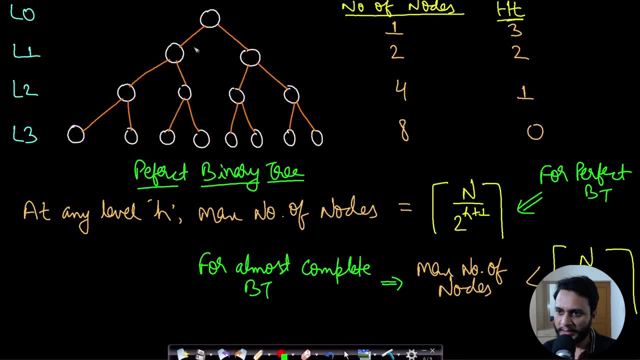 order of n. we will look at the proof. So before seeing at the actual proof, we will take an example. In this case, let us assume that we are taking a perfect binary tree And this is having four levels, that is, height from zero to three. Okay, Now I have already written the number of. 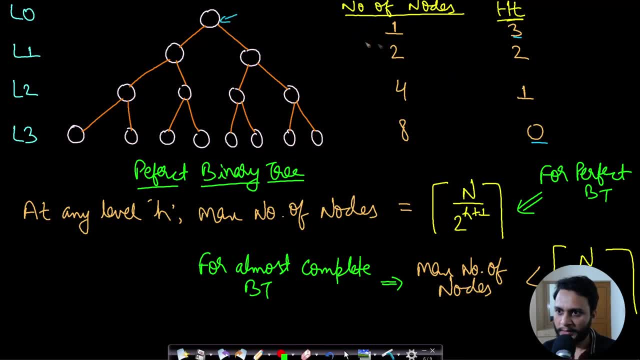 nodes here at each level. at level one, number of nodes will be one. this is the maximum number of nodes. this is a perfect binary. at level two, that is this: height two. okay, at height two, maximum number of nodes will be two. at height one, maximum number of nodes will be four. and at height 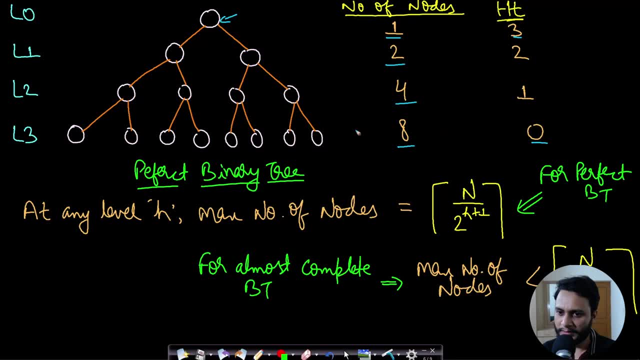 zero. maximum number of nodes will be eight. Okay, this is just an example. Now, at any level h, you will see that maximum number of nodes will follow this formula n by two to the power h plus one seal. Okay, so this is valid for perfect binary tree. you can take some other examples. 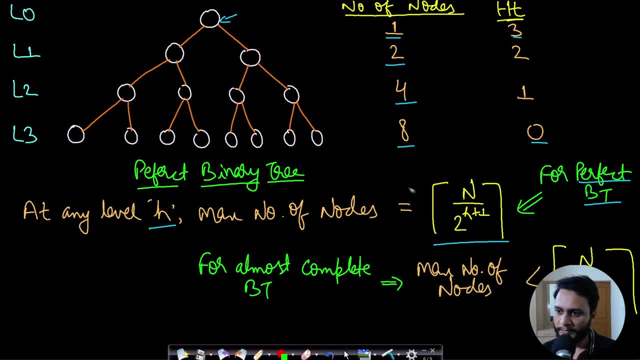 some other perfect binary trees and this formula will fit there. Okay, So what is h, h is nothing but the given height, And what is n, n is the number of nodes. Okay, So for almost complete binary tree, all the levels will not be entirely filled And therefore it will be having. 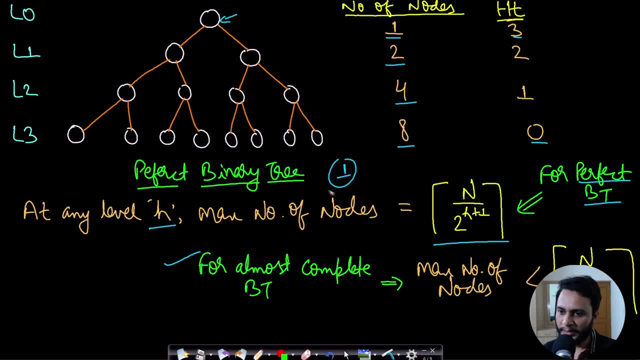 at least one node less than this perfect binary tree. So these all concepts I have already explained in my previous videos, so do watch it. the link will be given in the description below. So the maximum number of nodes in this case will be at least one less than what we have for the. 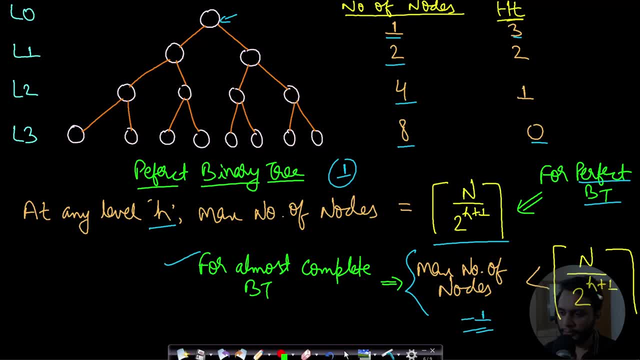 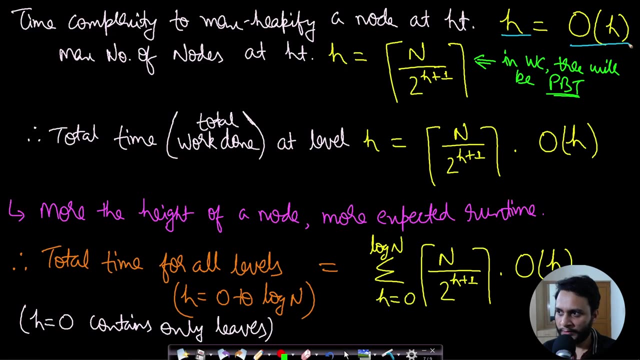 perfect binary tree and therefore it will always be less than n by two to the power h plus one seal rate. So I hope you got this concept. you can take some examples and just dry run, you will understand it better. So the time complexity to max CP phi, a node at height h, will obviously be order of h And in this 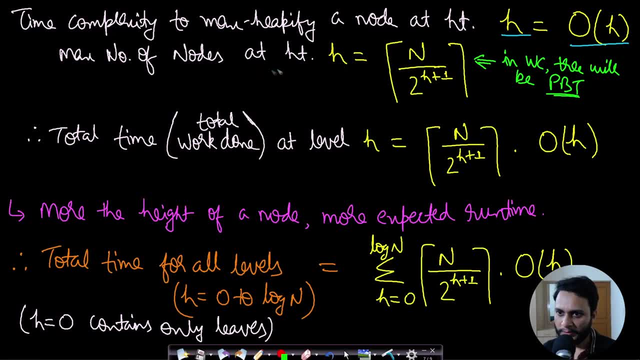 case h is nothing but log n rate. So the maximum number of nodes at a given height, h, is n by two to the power h plus one which is for the perfect binary tree. So in the worst case our complete binary tree will be a perfect binary tree. Therefore, the total time that is, you can also 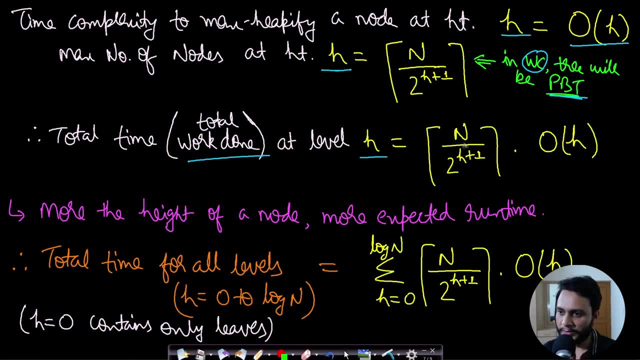 assume, as the total work done at level h will be equals to n by two to the power h plus one, seal into n by two to the power h plus one. So this is the maximum number of nodes at a given height. h order of h. because at a given level h you are having these many number of nodes And for each 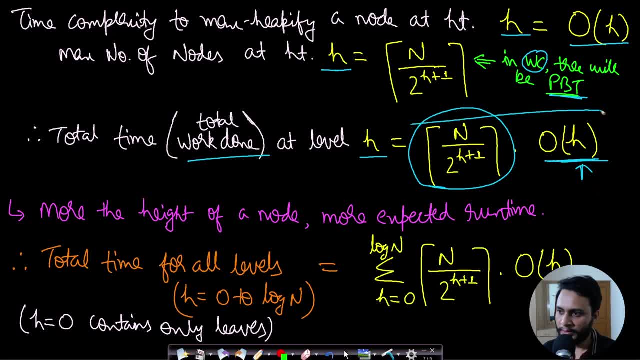 node, you will require this amount of time. So this will be the total time in order to heapify all the nodes at a given level. right Now. more the height of a node, more is the expected runtime because we need to move more and more downwards. In the worst case, we will have to move to the 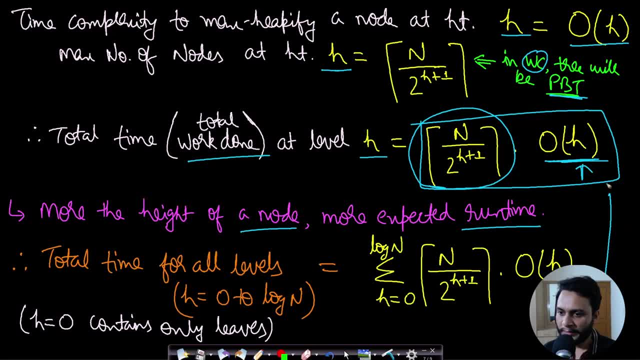 farthest leave. So if you are at a more height then we might be required to move a larger distance. So the time complexity will be higher if the node is at a greater height. So this is pretty logical. Therefore, the total time complexity for all the nodes, for all the heights, 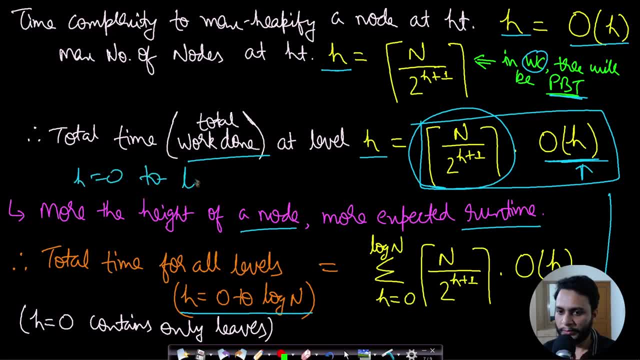 So our height will range from h equals to zero to log n, because this is the maximum height rate. So the total time will be ranging from h equals to zero to log n. summation of all the time for all the levels. And at each level we will be having n by two to the power, h plus one number of. 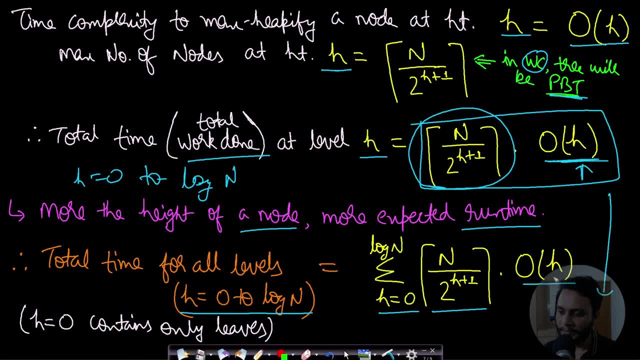 nodes. this is seen and that will be multiplied by the time complexity at each level. Okay, so this we had already understood And we are just adding for all the levels from h equals to zero to log n. Now, one thing to remember here is: h equals to zero is nothing but the last level, and the last level. 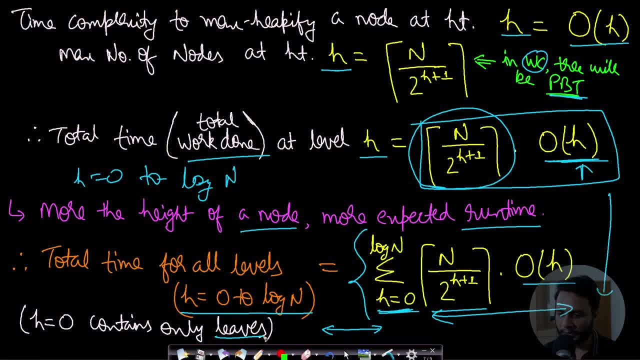 will obviously always be containing the only the leaf nodes, And we already know that the leaf nodes will always be following the min or the maxi property, So you don't really need to heapify the leaf nodes. So what we can do is we can start this- h equals to one- to log n. But 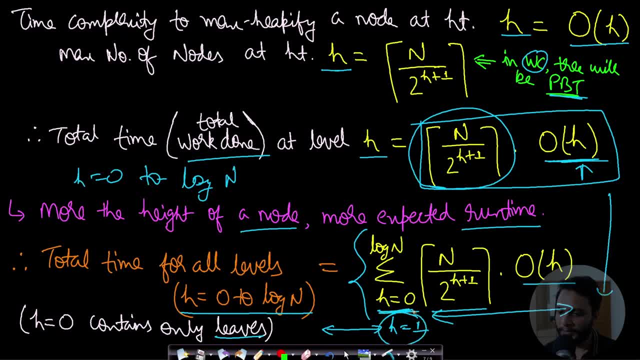 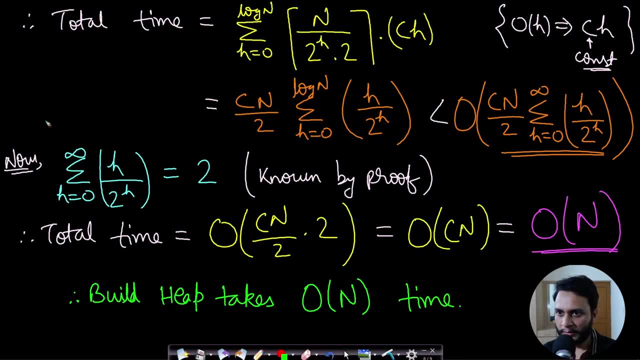 just for the sake of taking the worst case scenario, we will be taking from h equals to zero to log n. right Now, as you can see, we can just reformulate that formula which we had already written and write: total time equals to summation of h equals to zero to log n, And this will be n by two to the power h. 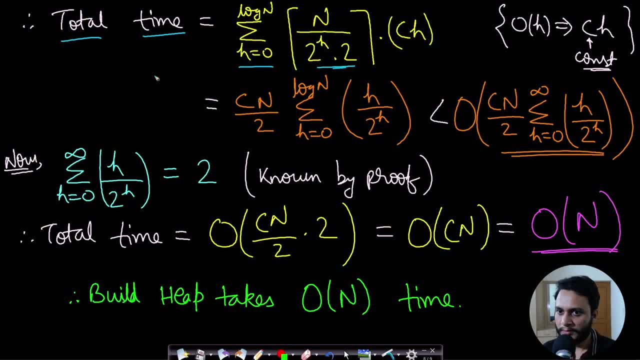 into two, into ch. So this was written earlier as two to the power h plus one and we can write it as two to the power h into two, and order of h can be written as ch, where c is a constant right. So if we again reformulate it then you will see that this n and c are 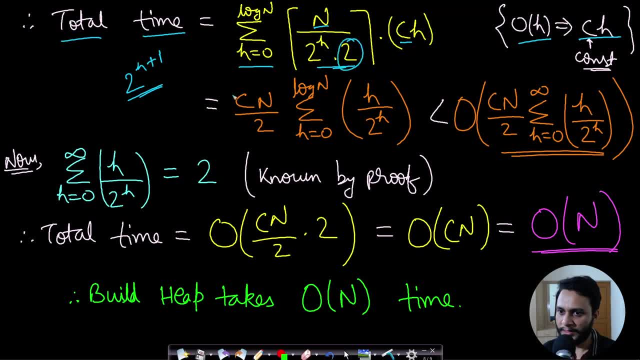 constant, so we can take it out. this two is also a constant, we can take it out, and whatever is left inside, because this is a variable of h. okay, So we are basically summing from: h equals to zero to log n, so variable is h here. 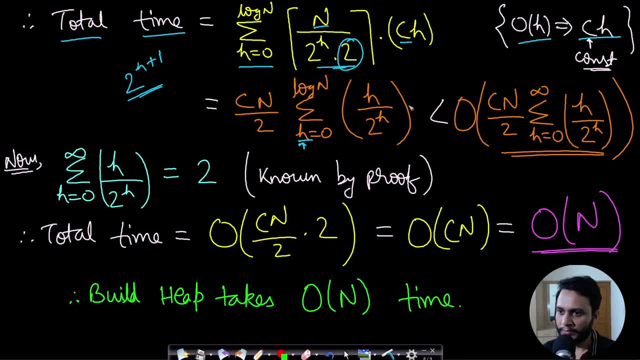 So, apart from match, everything else will be going out, so this will remain right now. this is pretty logical: that whatever you are seeing here will always be less than whatever you are seeing here, because all the variables are same. everything is same, but except this summation is running from H equals to 0 to infinity, and since this, H and 2 to the power. 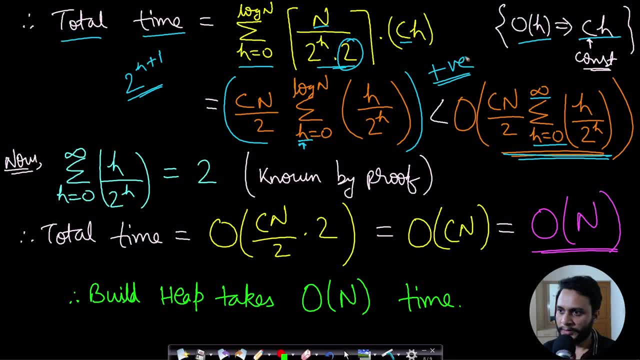 H is always positive. therefore, if you are adding positive numbers more number of times, then obviously it will be greater. therefore, this right hand side will always be greater than this left hand side. okay, now it is already known by proof that summation H equals to 0. to infinity H by 2, to the power H will be equals to 2. this you can find on internet. 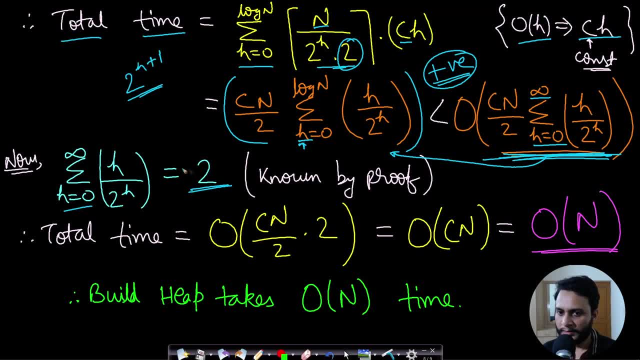 if you are interested in knowing about this. therefore, once we know this, then obviously the total time For this one, for this case, will be: equals to Cn by 2- is already like a constant value- and this total summation of H equals to 0, to infinity, H by 2, to the power, H will be.